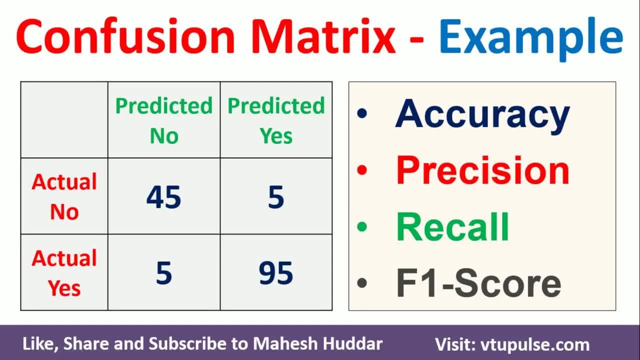 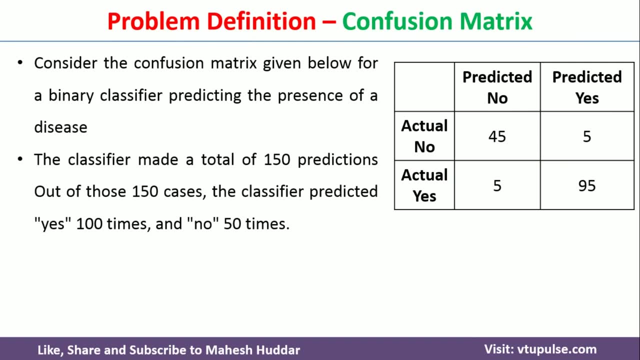 Welcome back. In this video I will discuss how to find the different performance metrics, like accuracy, precision, recall and so on, given the confusion matrix. In this case, we have been given a confusion matrix with 150 predictions Out of 150 predictions. there are 100 examples. 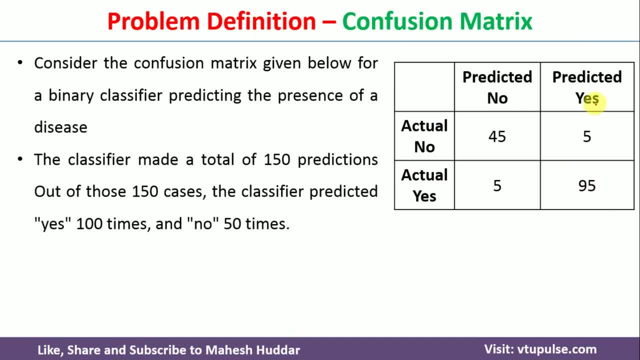 where class classified or predicted as yes in this case, and 50 examples were predicted as no in this particular case. And out of 150 examples there are totally 50 examples are of type no and 100 examples are of type yes. Now, given this particular data, we need to find 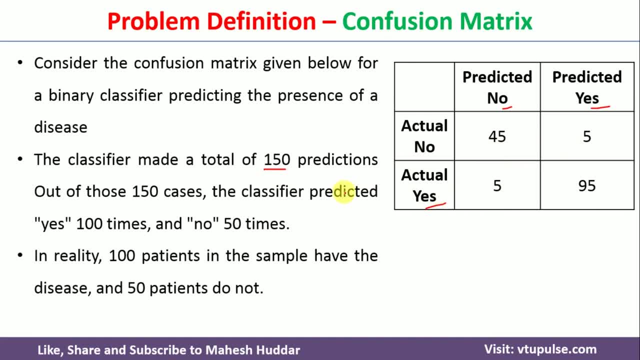 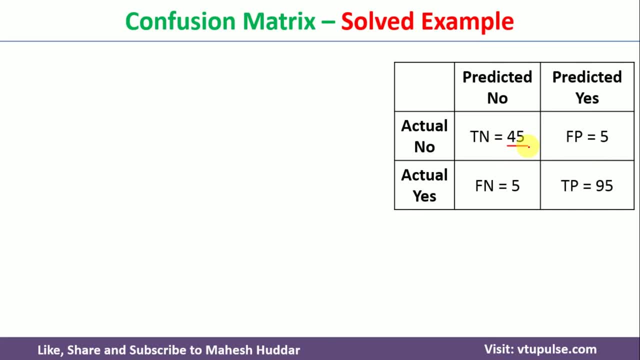 the different performance metrics of this particular classifier. So first we will try to give some names to each of these particular numbers. Now, if you look at this particular 45, these 45 examples are of type no. actually, When you look at this particular 45, this 45 examples are of type no. When you look at this: 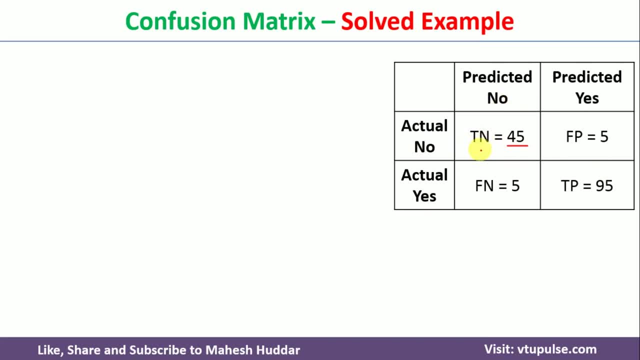 they were predicted as no here, so that is the reason you can say that it is a true negative in this case. and coming back to this particular 5, these 5 examples are actually of type no but predicted as yes over here, so you can say that these are false positive actually. 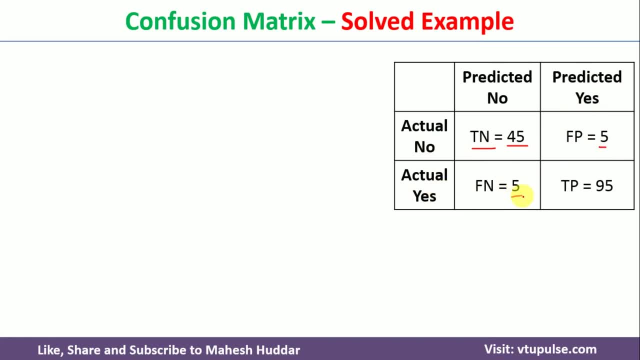 now coming back to this one, this particular 5 are actually of s type but predicted as no. here the meaning is it is false, negative. and this particular 95 examples are of type yes and they were predicted as yes over here. so you can say that it is a true positive in this case. 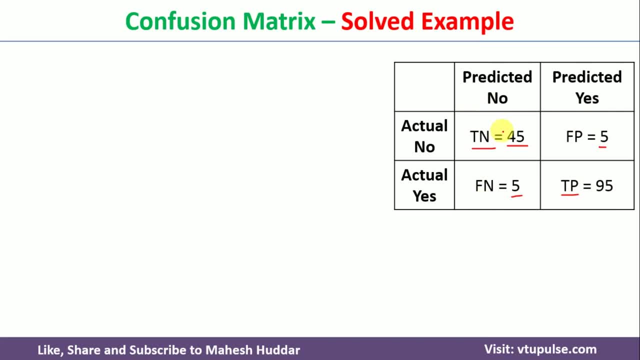 so, given this particular data, we will try to find out the first performance matrix, that is the accuracy. accuracy is the overall correctness of this particular model over here. so that is equivalent to the total correct predictions, that is, the true negative plus true positive divided by total number of predictions over here. so that is true positive and true negative is. 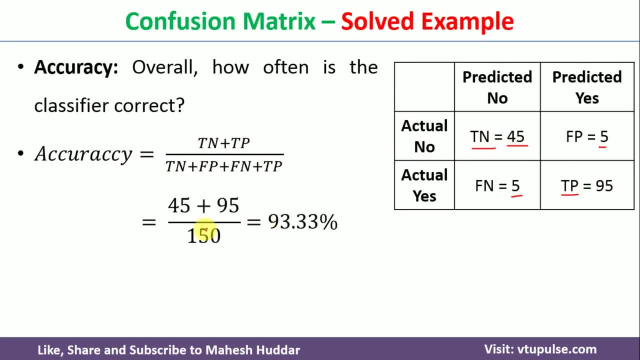 equivalent to 45 plus 95 over here. divided by total number of examples are 150 and if you calculate this particular equation you will get 93.33 percent over here. that is the accuracy of this particular model in this case. coming back to the next performance matrix, that is, the misclassification rate, the. how often? 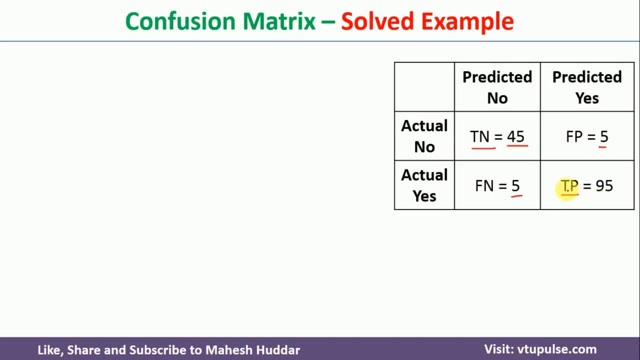 were predicted as yes over here, so you can say that it is a true positive in this case. so, given this particular data, we will try to find out the first performance matrix, that is the accuracy. accuracy is the overall correctness of this particular model over here. so that is. 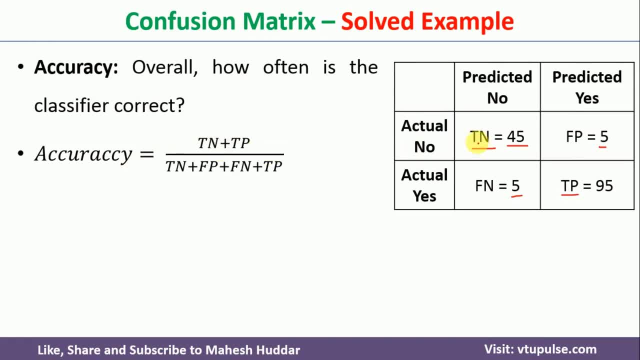 equivalent to the total correct predictions, that is, the true negative plus true positive divided by total number of predictions over here. so that is true positive and true negative is equivalent to 45 plus 95 over here. divided by total number of examples are 150 and if you calculate this particular 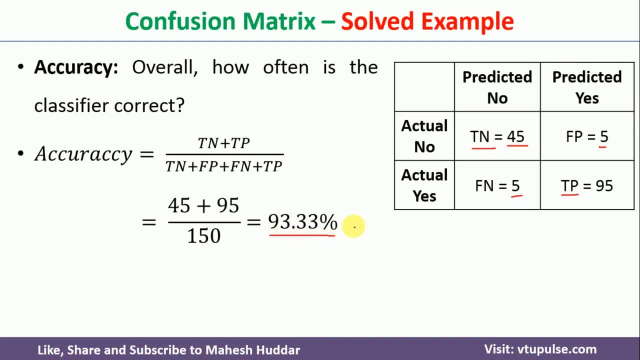 equation, you will get 93.33 percent over here. that is the accuracy of this particular model in this case. coming back to the next performance matrix, that is the misclassification rate, the how often the classification was done wrong in this particular case. that is the total misclassification. 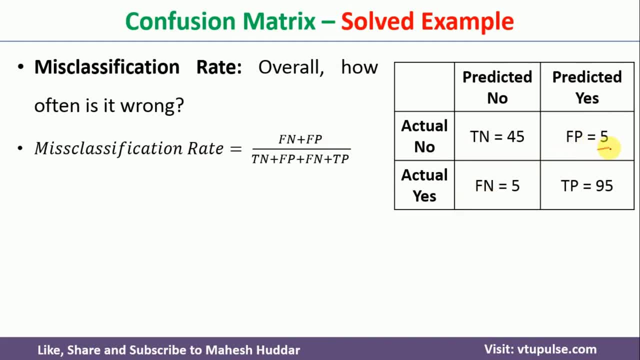 divided by total number of examples, that is this: five examples are of type no and they were predicted as yes here. that is the misclassification. and this particular five examples are of type yes, but they were predicted as no here. that is nothing but fn plus fp divided by total number of examples. here, that is 10 divided. 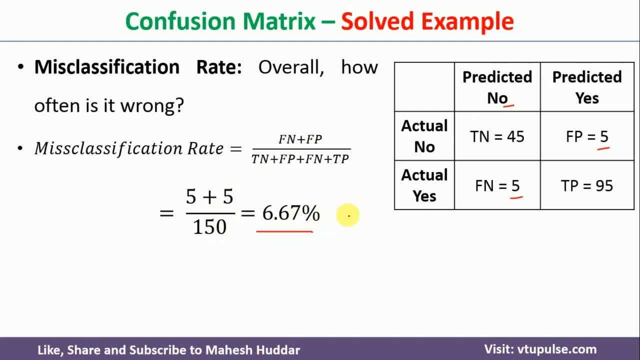 by 150, that is equivalent to 6.67 percent over here. the next performance matrix is true positive rate. that is nothing, but when a particular example is yes and how often that example is predicted as yes over here. so in this case the total s examples are 100 and the total 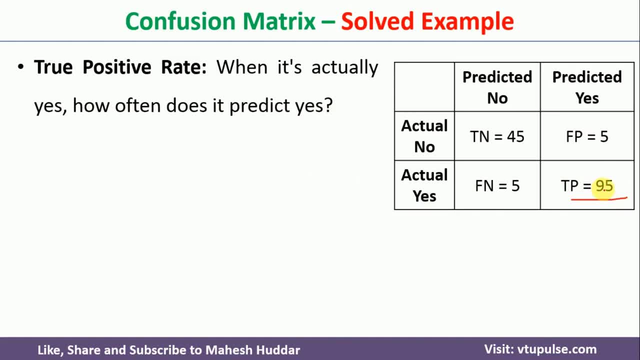 number of times it is predicted as yes is 95 over here. so this will be tp divided by actual s examples over here. that is 95 divided by 100 in this particular case. so it is also called as sensitivity or recall. if i put those particular values in this particular case, i will get 95. 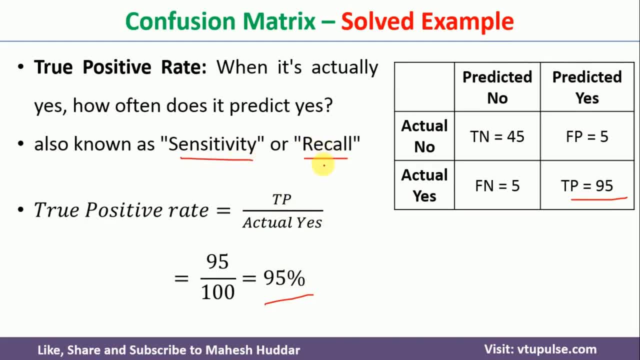 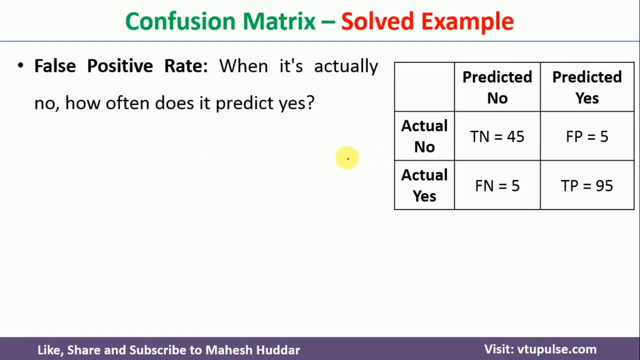 percent of true positive rate or sensitivity or recall, in this particular case, coming back to the next one, that is a false positive rate. that is, when a particular example is no, how often it is predicted as yes over here. so in this particular case, five times a negative example is classified as yes over here. that is nothing but 5 divided by 50 in this. 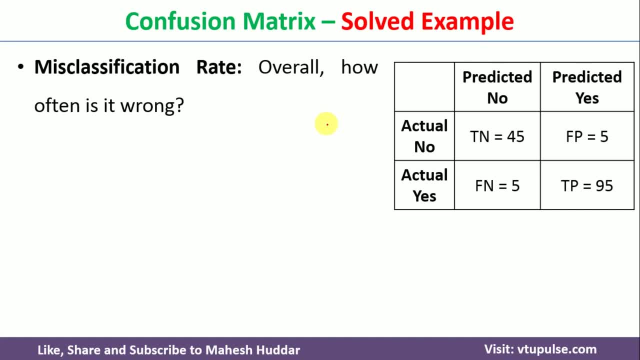 the classification was done wrong in this particular case. that is the total misclassification divided by total number of examples. that is this: five examples are of type no and they were predicted as yes here. that is the misclassification, and this particular five examples are of type yes, but they were predicted. 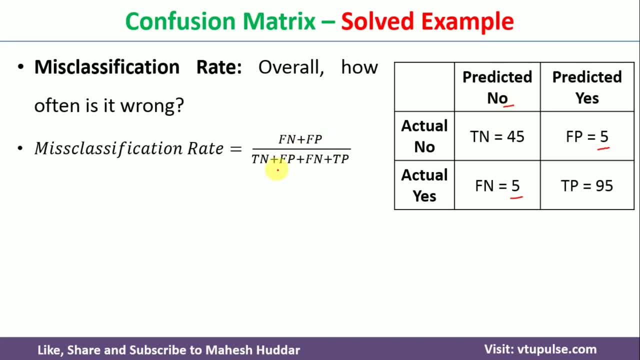 as no here, that is nothing but fn plus fp. divided by total number of examples- here that is 10. divided by 150, that is equivalent to 6.67 percent over here. the next performance matrix is true positive rate. that is nothing, but when a particular example is yes, and how often that. 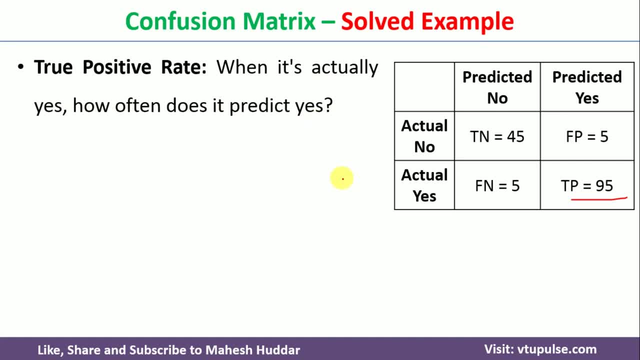 example, is predicted as yes over here. so in this case the total s examples are 100 and the total number of times it is predicted as yes is 95 over here. so this will be tp divided by actual s examples over here. that is, 95 divided by 100 in this particular case. so it is also called as: 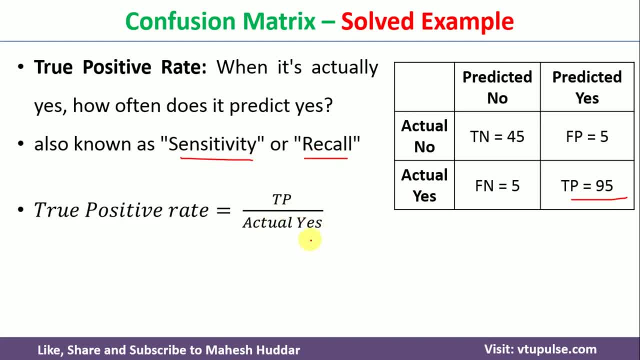 sensitivity or recall. if i put those particular values in this particular case, i will get 95 percent of true positive rate or sensitivity or recall in this particular case. coming back to the next one, that is a false positive rate. that is, when a particular example is no, how often it is predicted as yes over here. so in this particular case, five times. 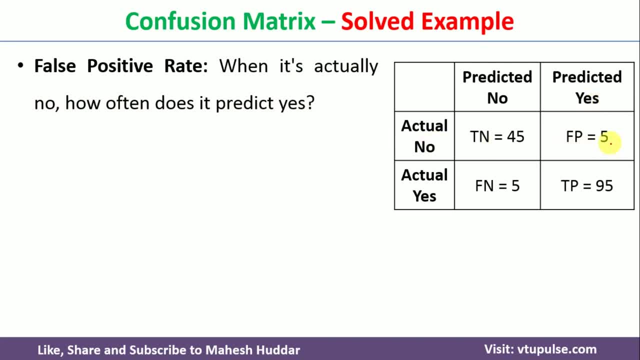 a negative example is classified as yes over here, that is nothing but 5 divided by 50 in this particular case, that is fp. that's a false positive divided by actual no in this case, which is equivalent to 10 percent over here. coming back to the next one, that is false positive rate. 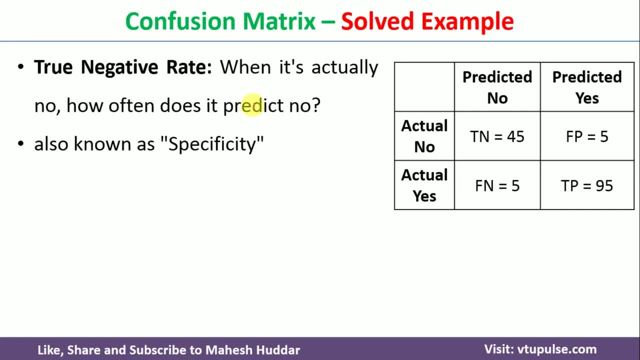 next one that is a true negative. that is when a particular example is negative. that is negative how often it is predicted as no here. so in this case it is predicted as no in 45 examples out of 50. so that's the reason you can say that true negative is 45 divided by 50. that is equivalent. 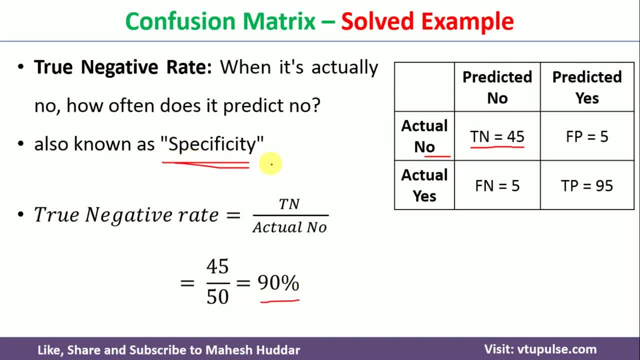 to 90, and it is also called as specificity. in this case, the next performance matrix is called as precision. this is nothing. but when it predicted as yes, how often it is correct- for example, in this case, 95 percent of the time or 95 times examples were classified as yes, and how often it is correct over here. so that is nothing. 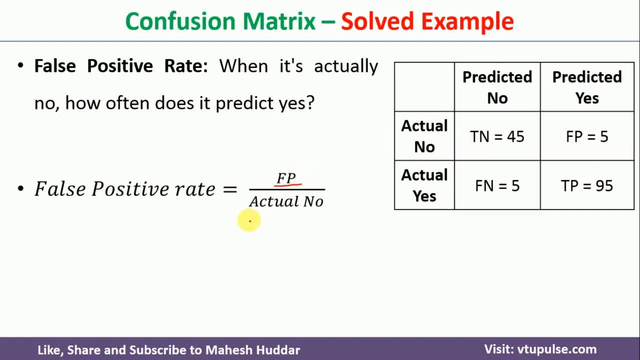 particular case that is fp. that's a false positive divided by actual no in this case, which is equivalent to 10 percent over here. coming back to the next one, that is false positive rate. next one: that is a true negative. that is, when a particular example is negative, that is negative. 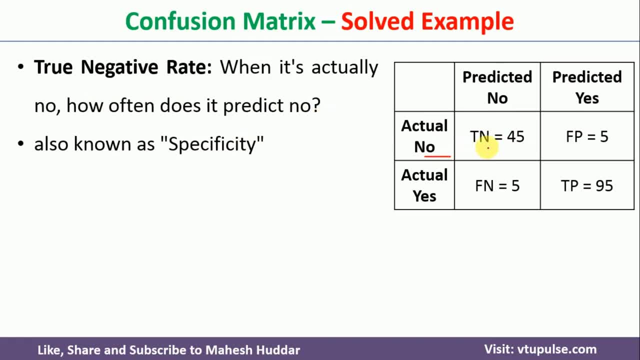 how often it is predicted as no here. so in this case it is predicted as no in 45 examples out of 50. so that's the reason you can say that true negative is 45 divided by 50. that is equivalent to 90 and it is also called as specificity in this case. the next performance matrix is called as: 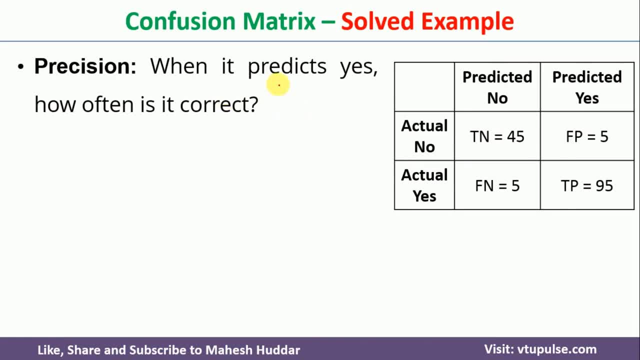 precision. this is nothing but when it predicted as yes, how often it is correct. for example, in this case, 95 percent of the time or 95 times examples were classified as yes- and how often it is correct over here. so that is nothing but the total number of uh yes predictions divided by uh, that is number of times the example is: 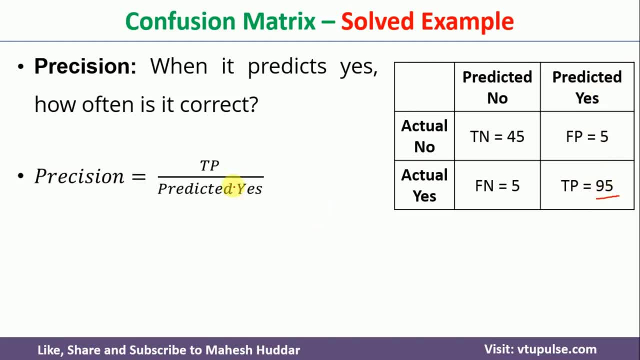 predicted as divided by total yes predictions over here, that is tp divided by predicted s over here, that is 95. divided by 100, again it is 95 percent over here. and the last one is something called as prevalence. that is nothing. but how often does yes condition actually occur in our sample? that is nothing but actual s. 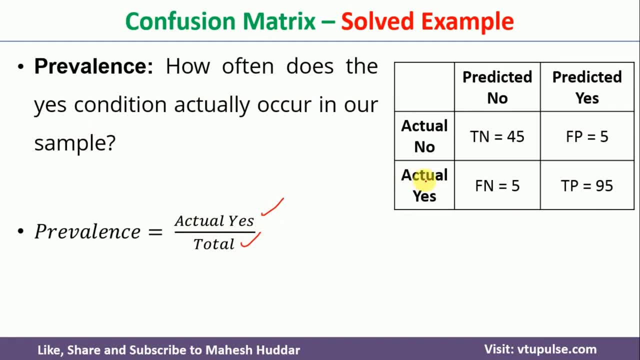 divided by total number of examples, actual s is 95 and actual s is actually 100. divided by total number of examples are 150 over here. that is nothing but 66.67 over here. different performance matrix we usually use in machine learning model to know the performance of that particular model. 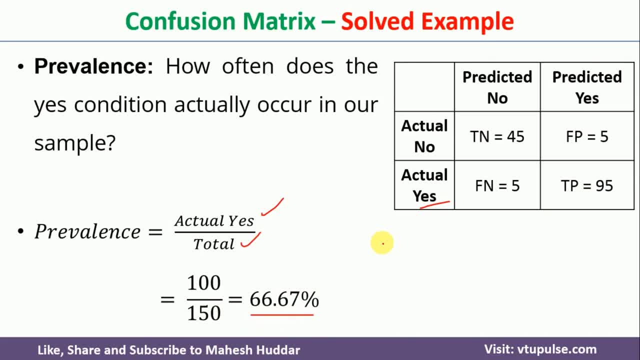 i have explained how to calculate these particular values with a simple example. i hope this particular concept is clear. if you like the video, do like and share with your friends. press the subscribe button for more videos. press the bell icon for regular updates. thank you for watching.